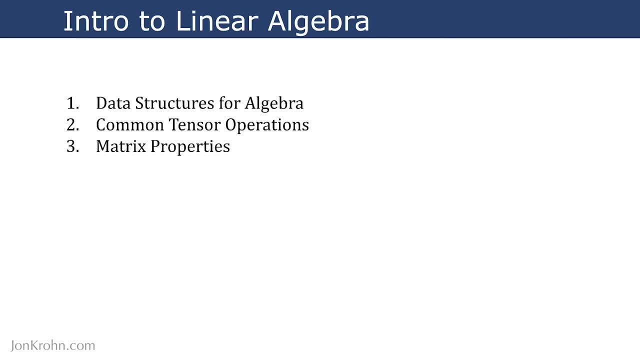 And finally, the final subject in this subject is matrix properties. We're going to kick off segment one in this video: Data Structures for Algebra. All of the topics in here are what linear algebra is, and then we're going to talk about linear algebra as a whole. So let's get started. 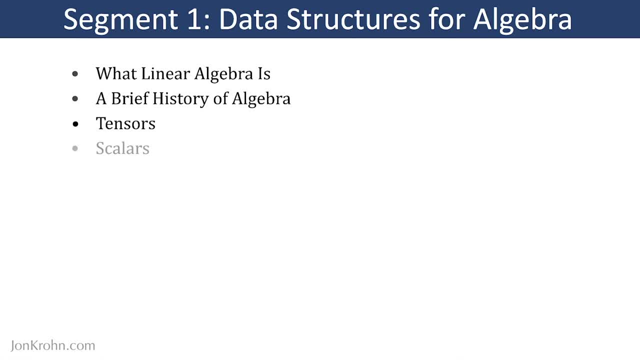 So here is a brief history of algebra: tensors, particular types of tensors, including scalars, vectors, simple manipulation of vectors, such as transposition, ways of characterizing vectors like norms, and special types of vectors like unit vectors. more special vectors: basic, orthogonal. 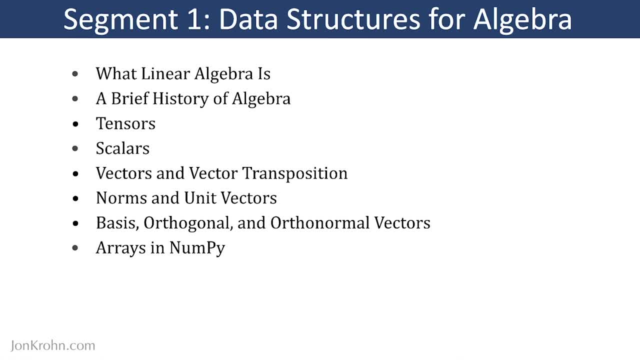 and orthonormal. We're going to tackle building vectors in NumPy and other types of tensors, as well as matrices and tensors more generally in TensorFlow and PyTorch, the two most popular automatic differentiation libraries. In this first video we're going to talk about what linear algebra is. 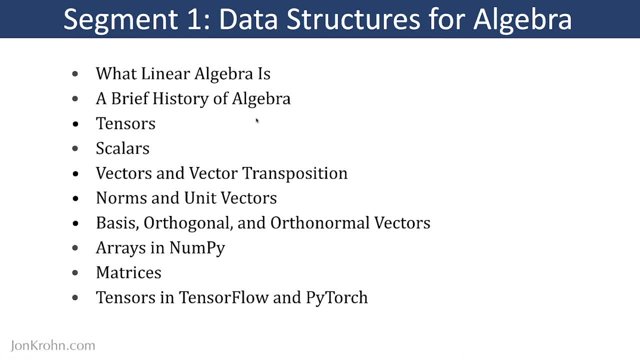 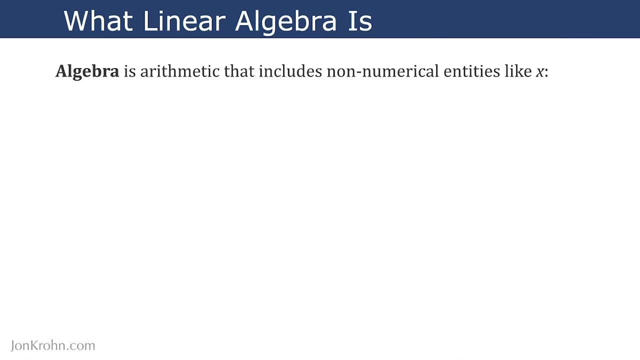 and just do a single slide on a brief history of algebra. You'll have to wait for future videos for the rest of the content. So what is linear algebra? Well, first let's talk about what algebra more generally is. So algebra is arithmetic. that includes any non-numerical entities like x. So here's a simple example. 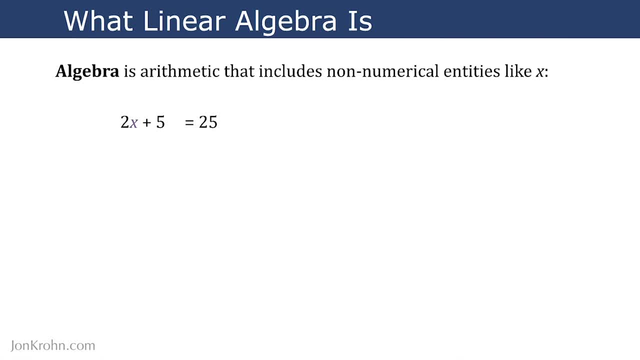 If we have this equation, 2x plus 5 equals 25.. Well, we can subtract 5 from both sides of the equation, and then that will leave us with 2x is equal to 20.. We can then divide by 2 on both sides. 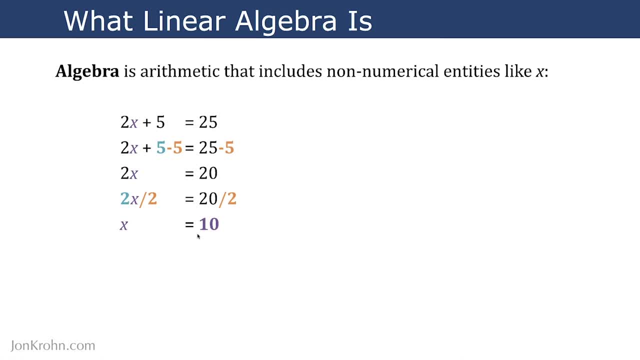 leaving us with 10 as our answer, And you can confirm for yourself that x must be equal to 10, because you can plug it into the original equation, and when x is equal to 10, 2x plus 5 comes out to 25.. It's the only solution to this equation. 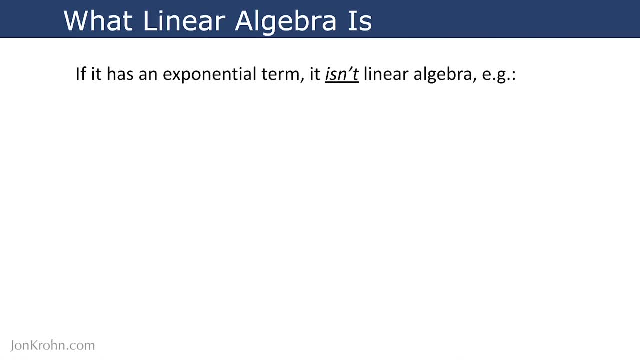 So that's what algebra is. Now to dig into what linear algebra is a bit more. it isn't linear algebra if it has an exponential term. So, for example, an equation that has 2x squared plus 5, well, that isn't linear. 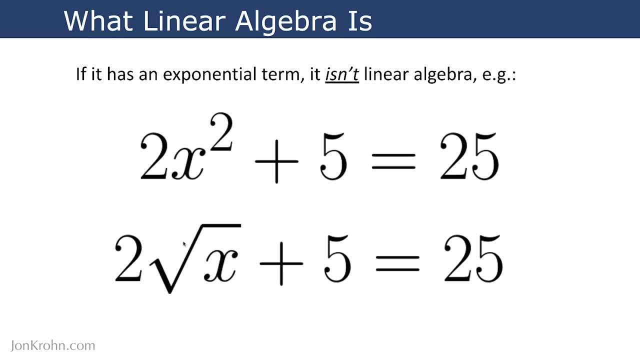 It's a non-linear transformation. And then a square root: that's also a non-linear transformation. So this equation is also not linear algebra. To give you a really nice and tidy definition of what linear algebra is, we could say that it's solving for unknowns within a system of linear equations. 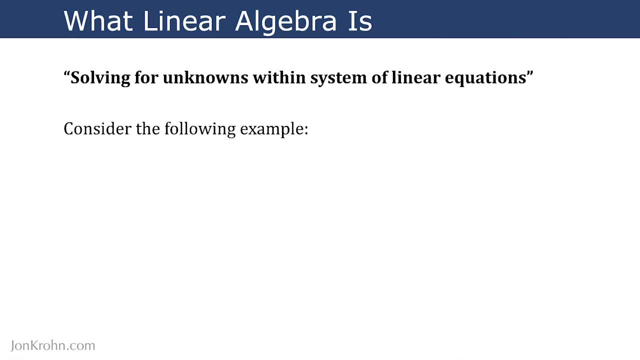 So let's talk about that idea of a system of linear equations, multiple linear equations, where we're solving for unknowns like x across several equations simultaneously. So here's an example. Let's say a sheriff has a car that travels at 180 kilometers an hour. 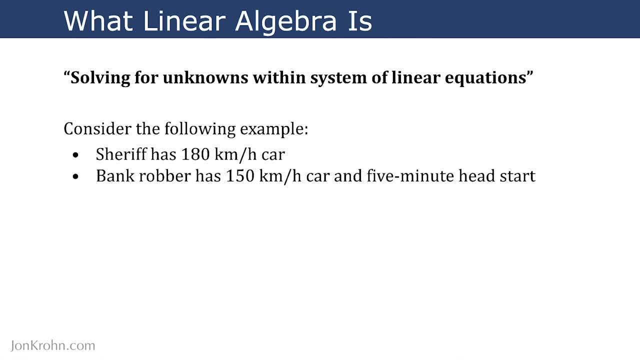 A bank robber has a slightly slower car. it goes 150 kilometers an hour, but that bank robber gets a five minute head start on the sheriff. So how long does it take the sheriff to catch the robber, And what distance will they have traveled at that point? For simplicity, let's ignore acceleration. 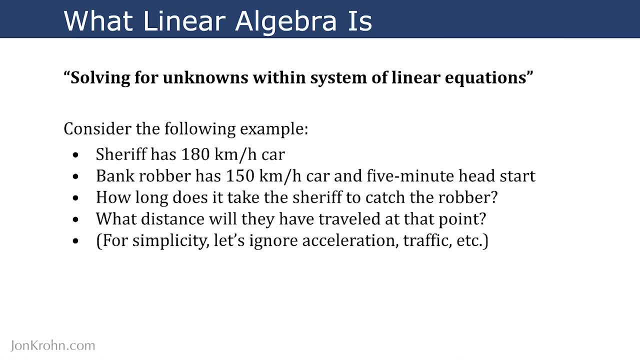 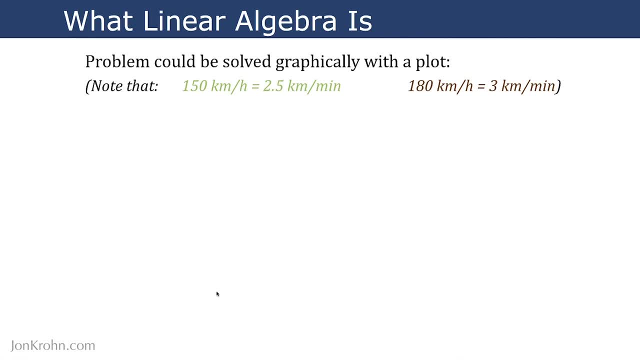 traffic etc. And we'll just assume that they're traveling in a straight line in one direction. So we can solve this problem graphically with a plot. We can note here that 150 kilometers per hour corresponds to 2.5 kilometers per minute. 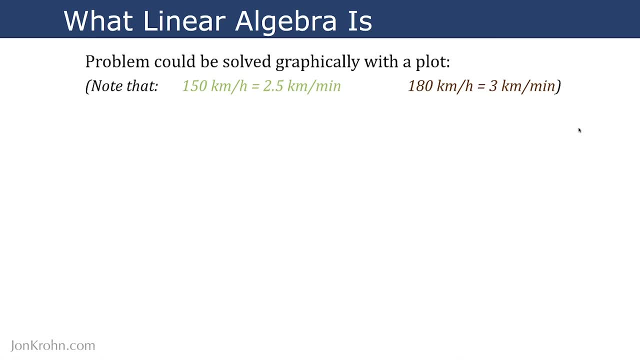 and 180 kilometers per hour corresponds to 3 kilometers per minute. You can plot things out here, And so we have a plot of time along the x-axis, the horizontal axis, in minutes, And then we have a plot of distance in kilometers. 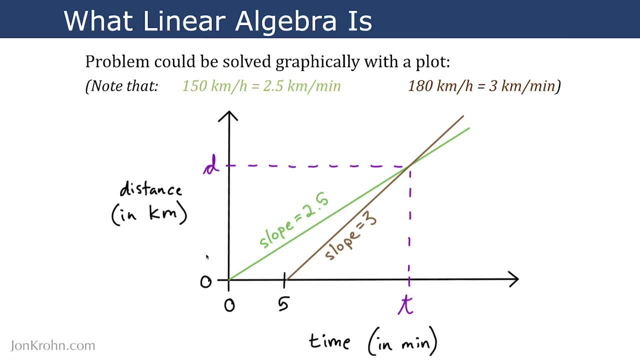 Along the vertical axis. You can see here there's a green line corresponding to our bank robber going 2 kilometers per minute. So that's a particular slope And our Sheriff is traveling at a faster speed so has more slope, a slope of 3 instead of 2.5,. 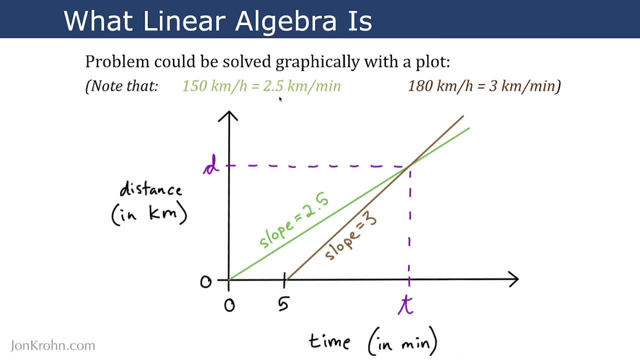 corresponding to 3 kilometers per minute instead of 2.5 kilometers per minute. And then we have a plot of time And we have a slope of 3 instead of 2.5, corresponding to 3 kilometers per minute instead of 2.5 kilometers per minute. 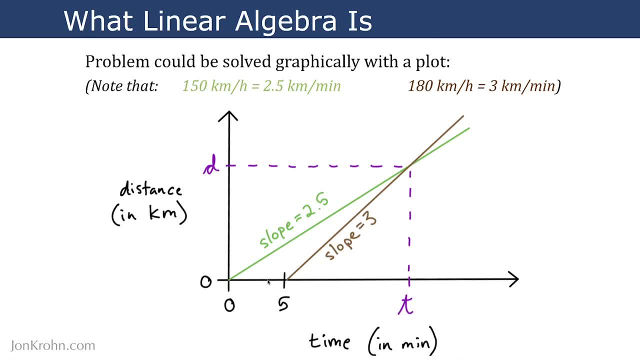 And then we have a plot of time And we have our 5-minute head start to the bank robber, accounted for by the gap here along the x-axis. So what we're trying to solve for is this crossover point where the sheriff catches. 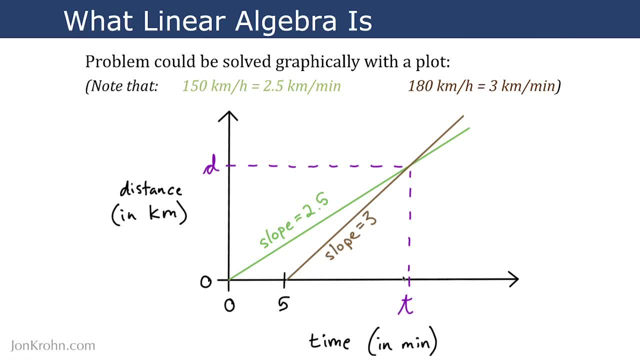 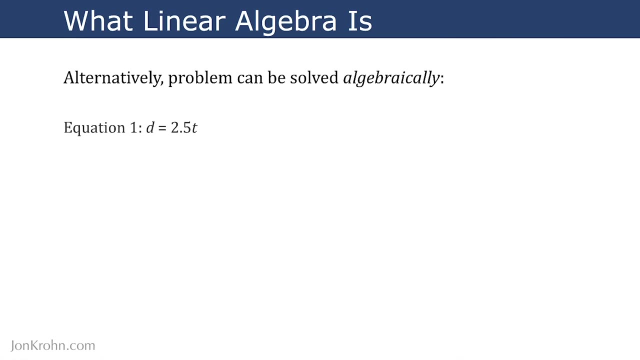 the bank robber. So what time is it, how many minutes have elapsed at that point, and what distance have they both traveled at that point? So you can see that graphically, you could come up with a solution here. Alternatively, we can solve the problem algebraically. 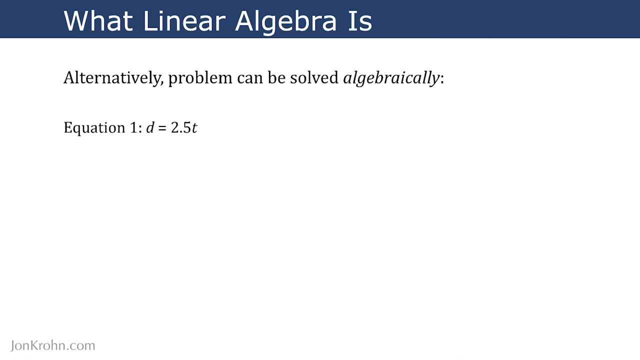 To represent the bank robber, we can have this first equation, which is distance d is equal to 2.5 times time, And then a second equation representing the speed of the sheriff. however, we also take into account that 5-minute head start. 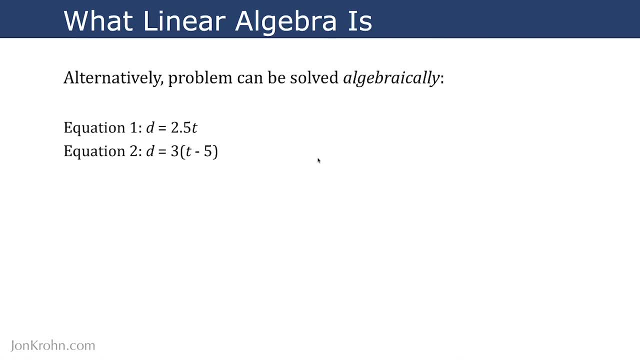 So we have a penalty of 5 for the sheriff. Now, both of these equations are equal to d, So we have a penalty of 5 for the sheriff. So we can actually set this term here equal to this expression here. So 2.5t is equal to 3t minus 5.. 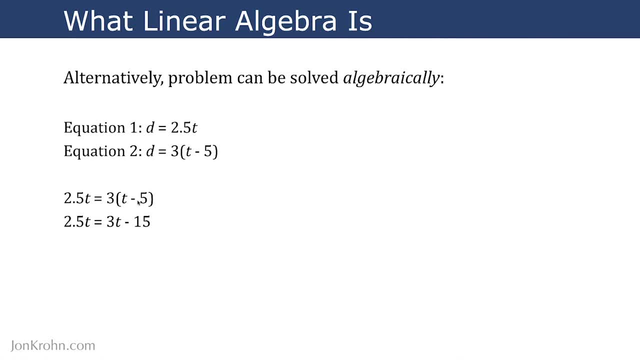 You can then multiply the 3 into the brackets to expand out this side of the equation, And then we start trying to isolate t by moving the d-axis. So we're going to do that by moving 3t over to the other side of the equation here. 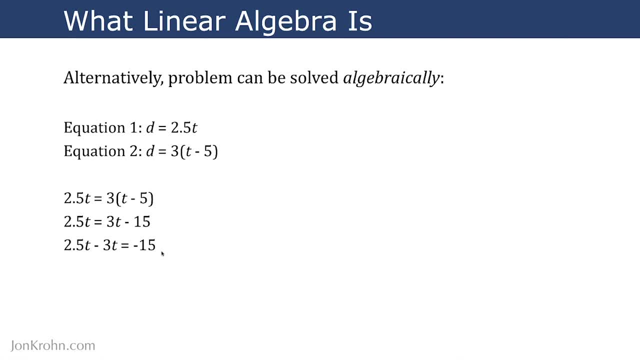 So we subtract 3t from both sides of the equation. When we do that now, 2.5t minus 3t gives us negative 0.5t is equal to negative 15. And so now we can divide both sides of the equation by negative 0.5. 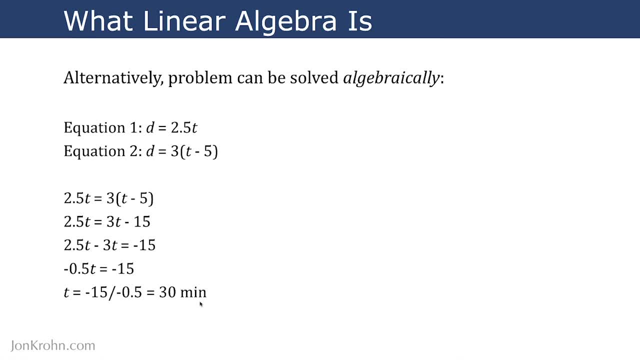 And that isolates t completely, giving us a time of 30 minutes. So now we know how long it takes for the sheriff to catch the bank robber. To figure out distance, this is really easy. now that we've solved for t, We can simply plug that 30 into the t in either equation. 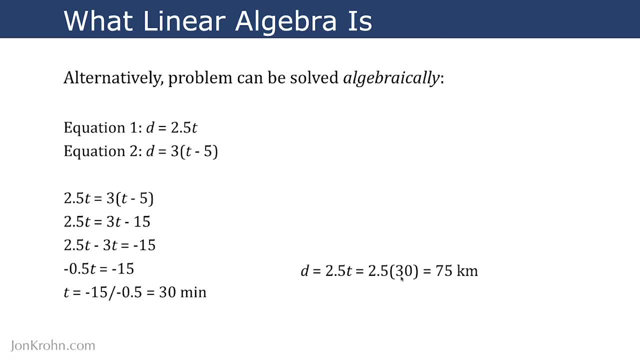 So for the first equation: 2.5 times t, 2.5 times 30 is equal to 75 kilometers, And then we can plug it into the second equation too. So 30 minus 5 is 25.. And 3 times 25 is 75.. 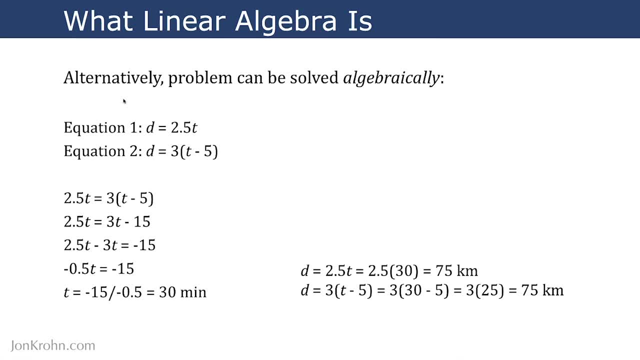 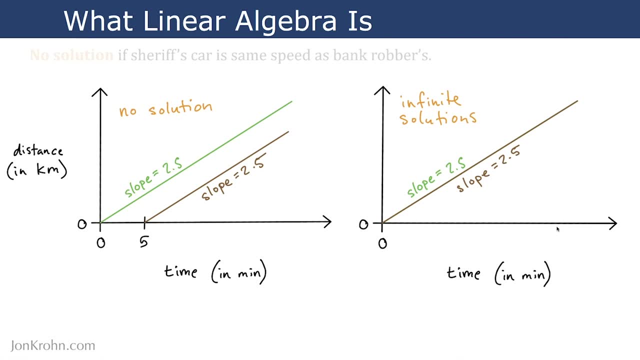 Of course, we get the same answer because it is a system of linear equations. Now, that was a nice, neat and tidy situation where we had one solution. However, there would have been no solution if the sheriff's car were the same speed as. 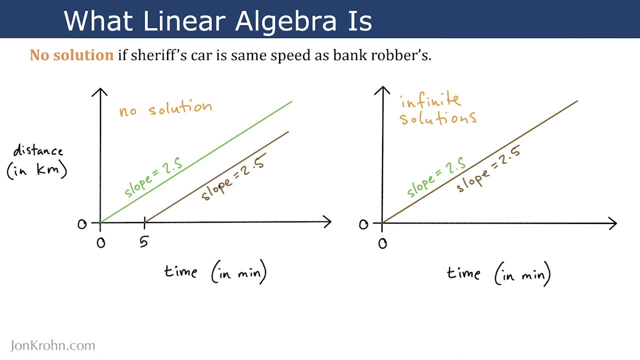 the bank robbers. So if they both were traveling at exactly the same speed forever, then there would be no solution to this problem. On the other hand, we could also have an infinite number of solutions if both the bank robber and the sheriff were traveling at the same speed and have the exact same starting 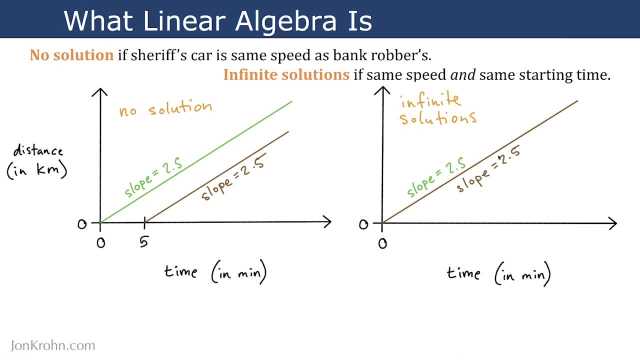 time. So the slope is the same, The start time is the same. now They overlap at every time point. These are the only three options in linear algebra, So you either have one solution, no solutions or infinite solutions. It is impossible for the lines to cross multiple times. 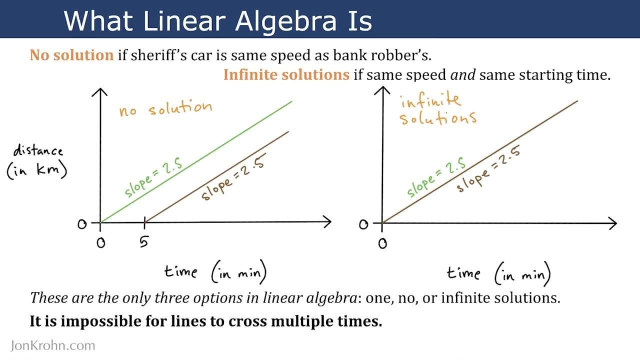 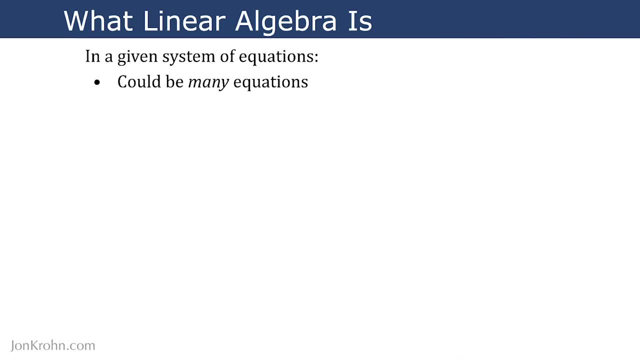 So this is a key part of this being linear algebra. in these systems of equations, In a given system of equations, there could be many equations. There could be many unknowns in each equation. In the example that I just showed you, there were two equations and there were two unknowns. 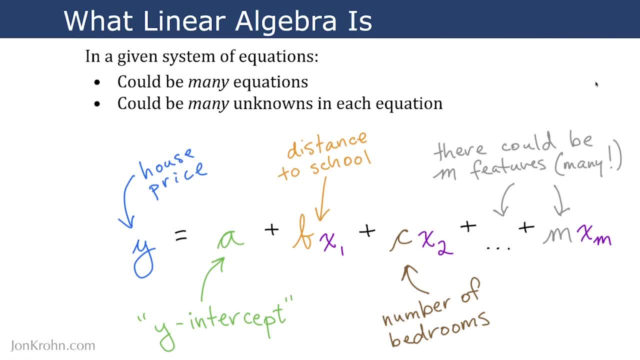 However, let's consider another example. here We are building a model. specifically, this is something called a regression model, which I'll get into a little bit of the detail here in case you're not already aware of it. In this model here, we are trying to predict house price. 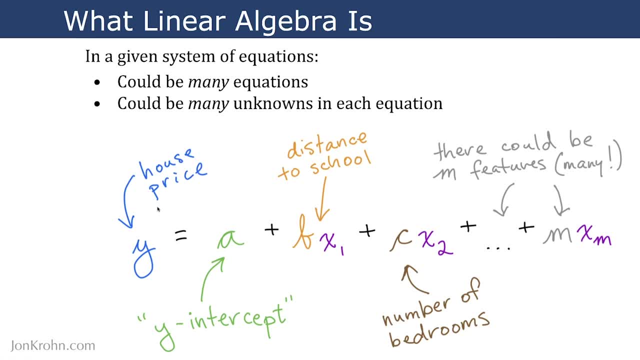 So we have for a given house, we have its price, that we're predicting y, And then we also have a number of features or variables that we are collecting To try to predict that house price And in a lot of cases, the more features that you have, the more accurately you're going. 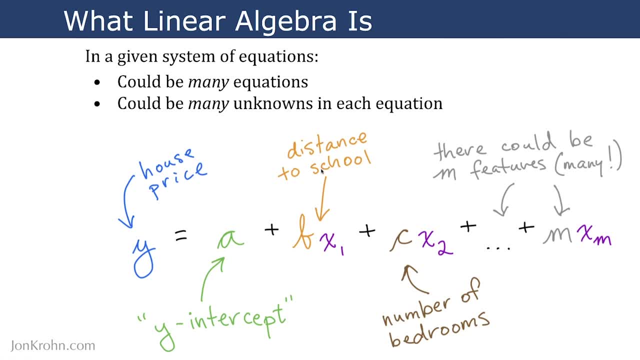 to be able to predict what you're trying to predict, the more relevant features. So some of the relevant features here might be distance to school or number of bedrooms and so on. I have m features here, And so b, c and m are examples of features. 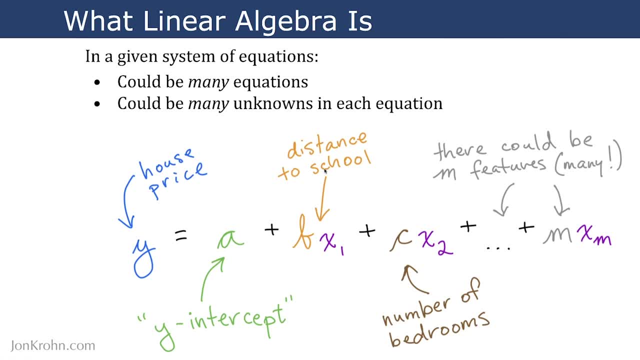 This could be an integer, the number three, distance to school. It could be a variable, It could be a value like 2.5, representing 2.5 kilometers, and so on. for however many features we have, in this case m features. 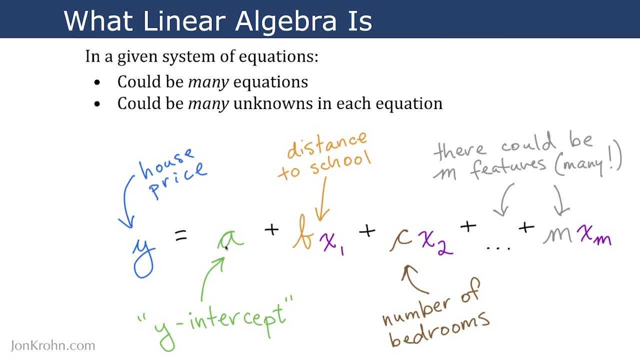 We also have to have a y-intercept here. So this is one last variable. It allows us to across all of the house prices that we have, have an average house price And without this y-intercept, without that kind of average baseline, before we start. 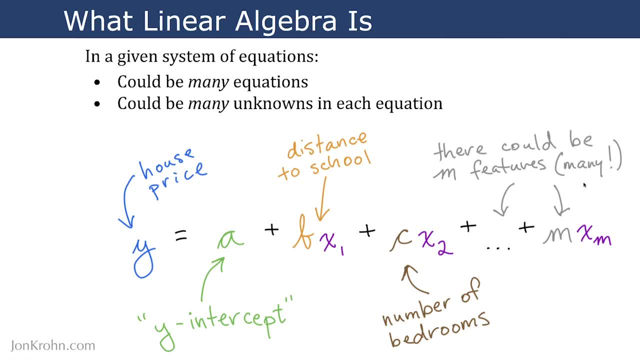 factoring in the other features, it becomes much more difficult to fit a good model. So here we have many unknowns and we could have effectively unlimited rows where every time we get a house price and collect the pertinent information associated with that house price, like distance to school, number of bedrooms and so on. that's another row. 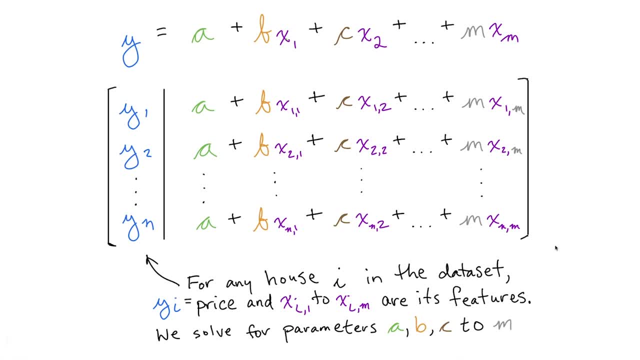 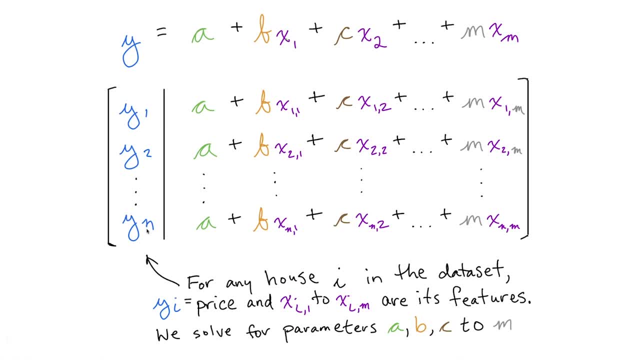 different houses, So n rows. We could have thousands of rows here And maybe a dozen features, So n can go up to 12 columns In a typical deep learning model. in contrast, it would not be uncommon to have millions of images, say for a machine vision model. 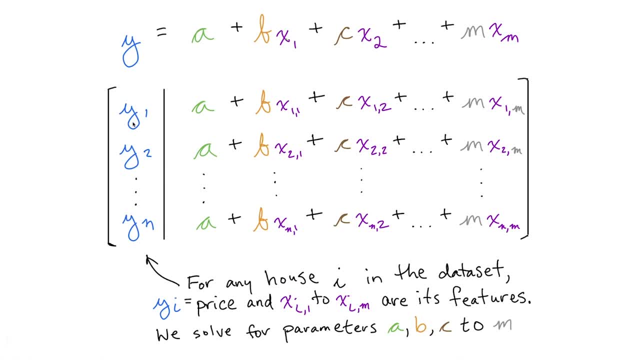 So we'd have millions of rows in our set of equations And millions of columns representing millions of parameters. potentially high resolution images would have a lot of pixels. So here's that equation from the preceding slide. I've now generalized it to a lot of different houses n houses. 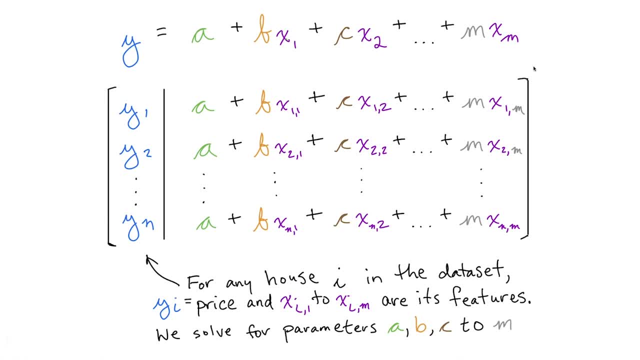 And I've made it into a set here using set notation from linear algebra, these square brackets, And so for any house, i in the data set, so we can call that particular price yi, which could be, say, $300,000, or what have you then xi1 to xim. 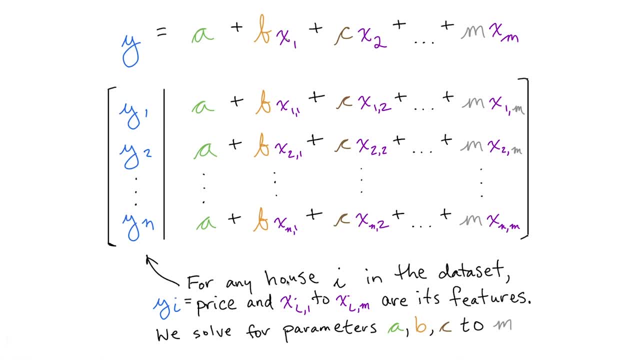 are all of the features for that particular house. i Now, across this whole system of equations we were trying to solve for the parameters a, b, c and m y. is our outcome that we're predicting, say, a house price? 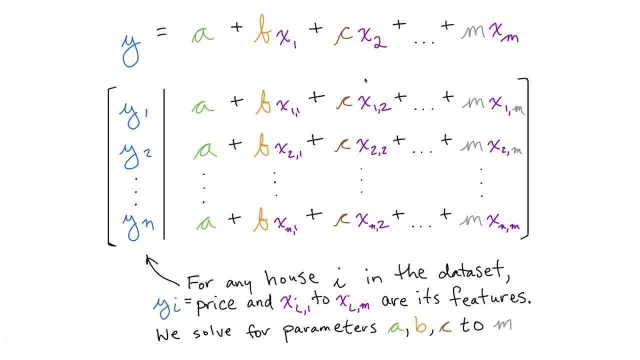 x is the variables, the actual values that we have associated with that house price. so x11,, x12,, x1m and so on, throughout this set of equations And these parameters, a, b, c and m. these are the unknowns that we're trying to solve for 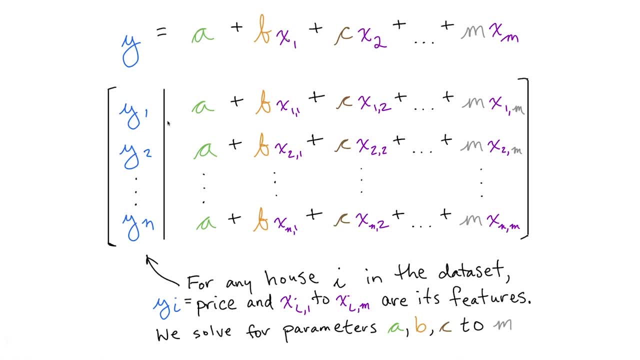 And you'll notice, these unknowns are consistent across all of the equations. So, whether we're talking about the first row, the second row, the nth row, a, b, c and m are going to be the same value. So we're trying to find an ideal value. 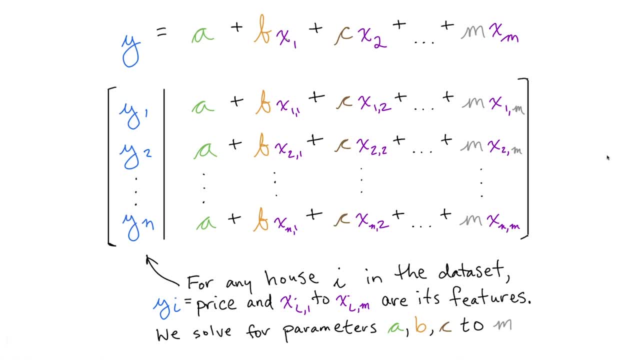 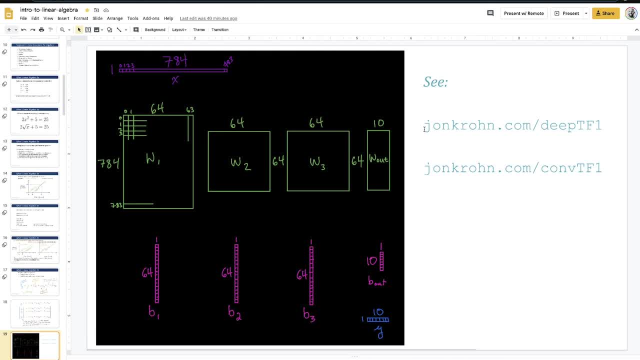 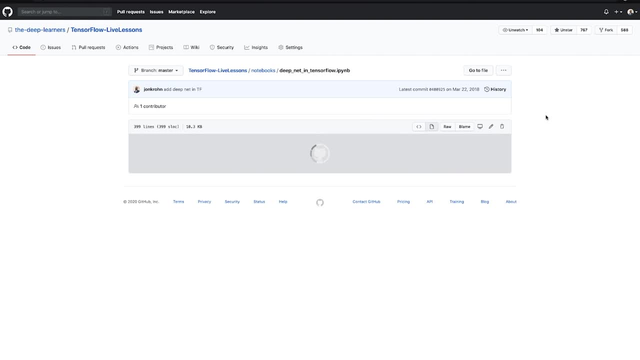 I have some data here And I'm going to use some quick examples to show you here of how this looks in practice. So if you go to johncroncom, slash deepTF1, this brings you to a deep neural network in TensorFlow. 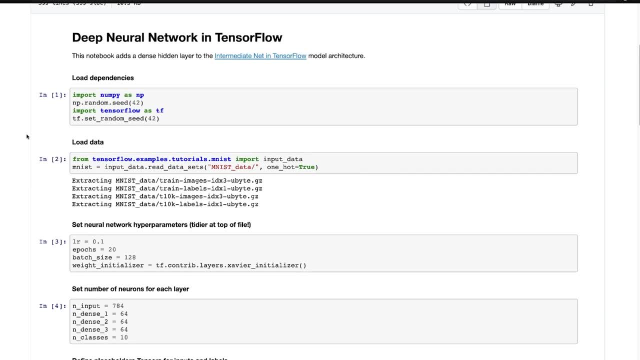 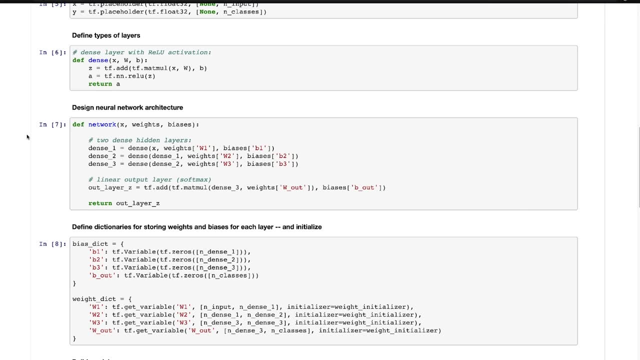 And by the end of this whole Machine Learning Foundation's journey, a lot of what's happening in this notebook will start to make sense Early on in this journey. I'm not expecting this stuff to make sense- The reason why I'm in here, though. 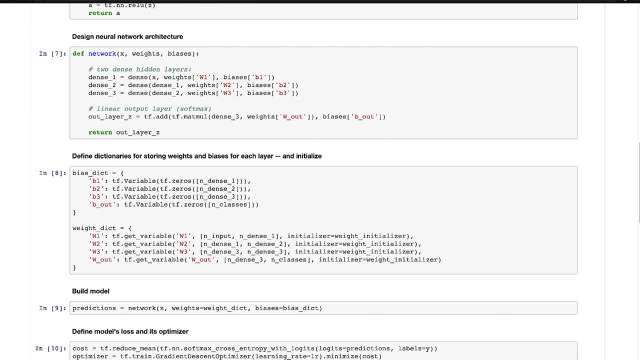 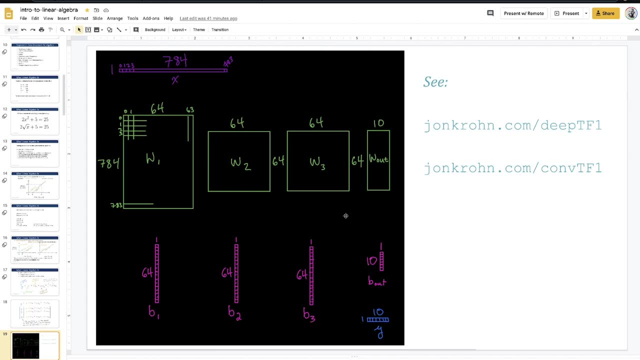 same kind of thinking that we had on the slides from linear algebra applies as well to various algebraic objects. What I'm going to introduce momentarily is tensors. So we have vector tensors here, one-dimensional tensors, and matrix tensors- two-dimensional tensors here. 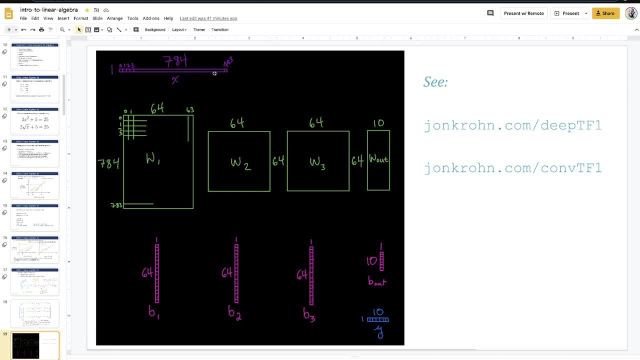 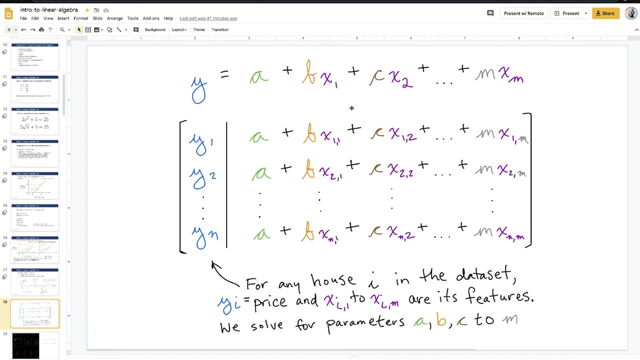 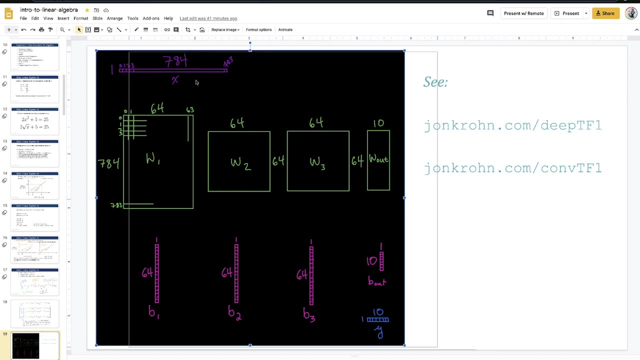 And so we have inputs. These x's are our inputs, just as they were in the preceding, pre-preceding example. So these x's are inputs into the model that we're using to predict the outcome: y In our deep learning model. in this particular model, it's a machine vision model. 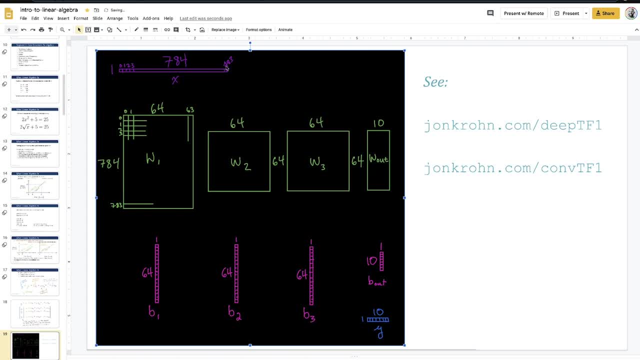 that's being passed in 784 pixels per image. So we have this vector of 784 pixels being input and we're using that to predict outcomes. is this y variable here, this vector of length 10, and in the middle we have these things called weights and biases: weights matrices and bias vectors. the specifics of that. 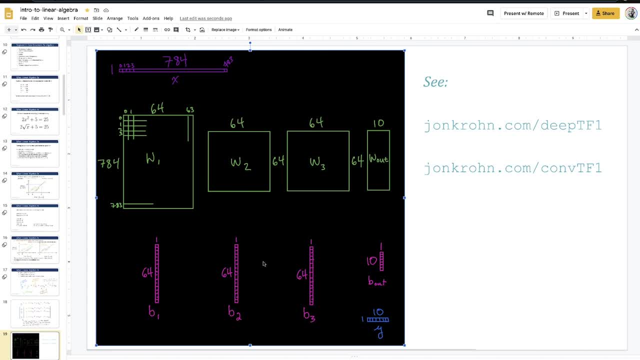 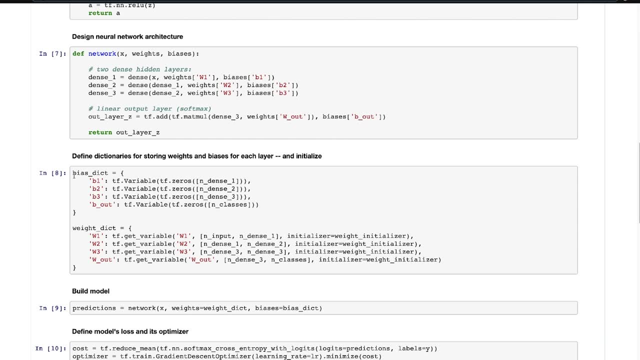 don't really matter, except that these are. i'm just trying to show you some linear algebra data structures, and these are encoded in whatever software language that we're using in this case. this is tensorflow here, and so we create bias vectors b1, 2, 3 and b out corresponding to b1- 2. 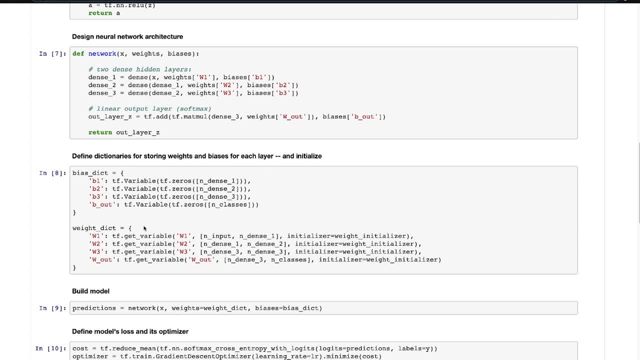 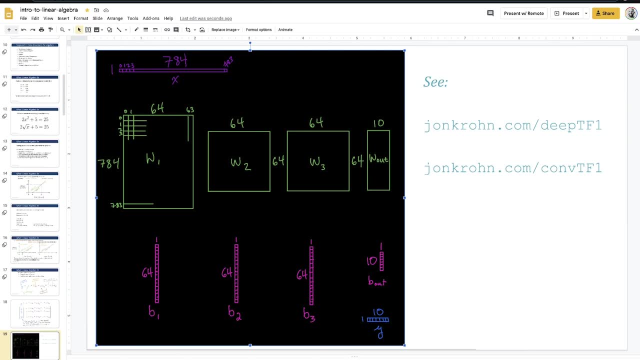 3 and b out these vectors here, and then we also have weights, so of a particular shape- w1, w2, w3, w out. so these are these matrices with these particular dimensions. so this is just an example of how we're going to have various you. 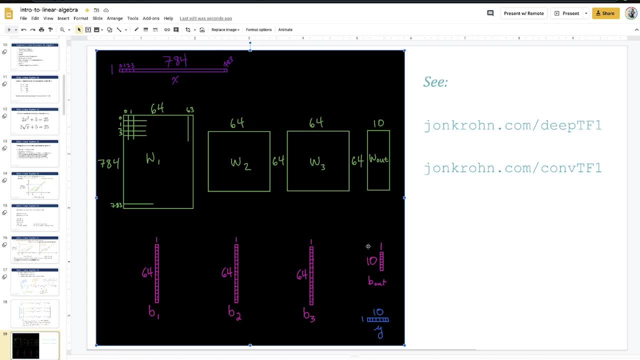 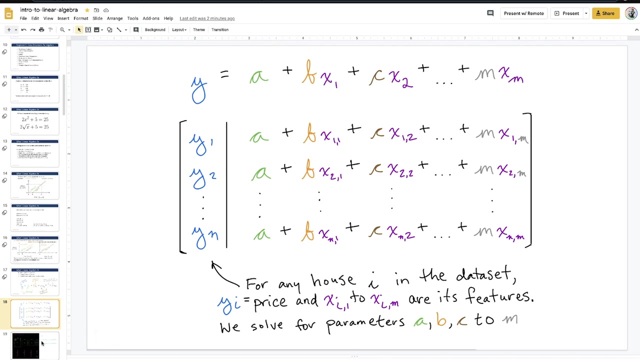 parameters- in this case weights and biases- that are going to be tuned by our machine learning algorithms in order to be able to map some particular pixel inputs into a prediction of what those pixels being input represents some particular outcome. so it's- this is just a slightly more complicated situation than we had with a linear regression example, and we can take it just. 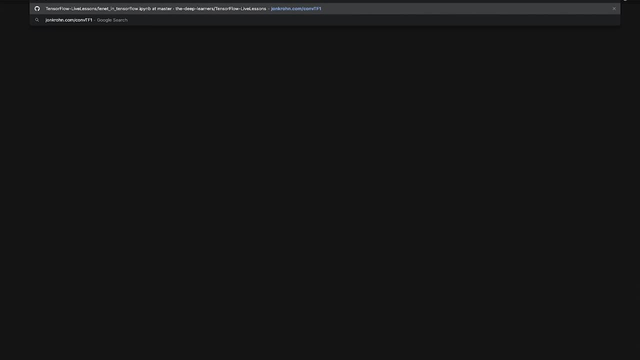 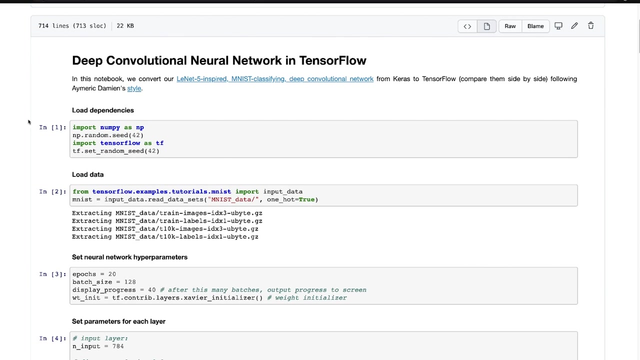 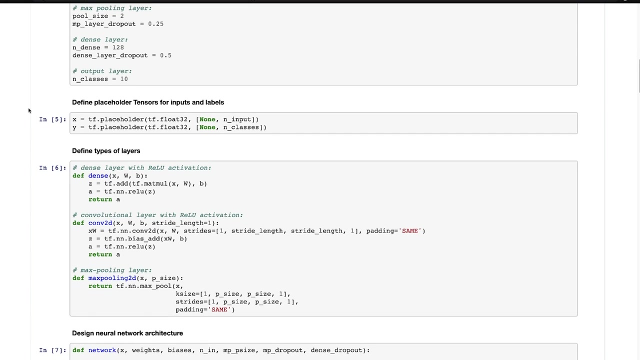 one step further by showing that these linear algebra objects don't have to be two-dimensional. we can have higher dimensional linear algebra objects, higher dimensional tensors. i'll explain all this terminology in more detail in the next video, but for now it suffices to say that we have these. 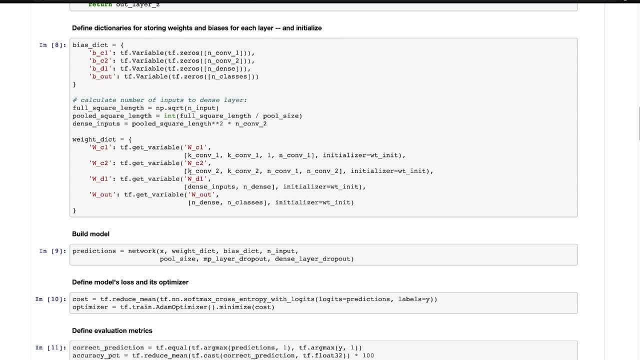 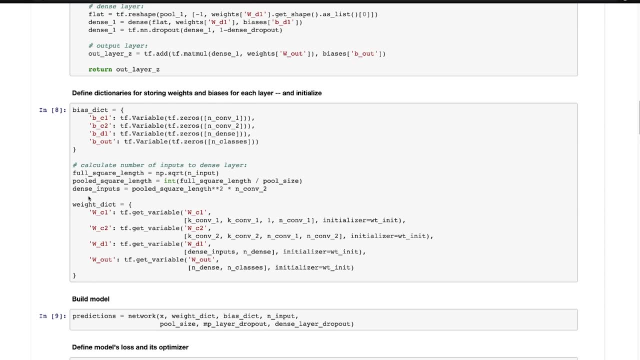 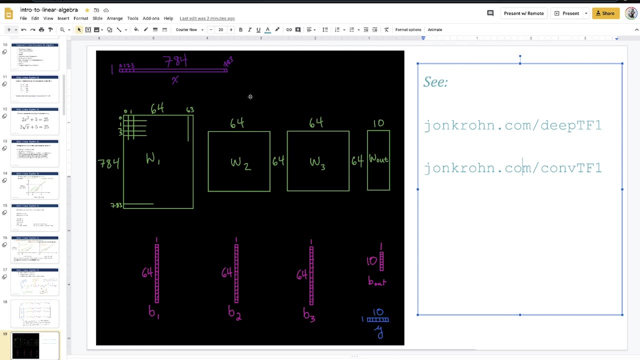 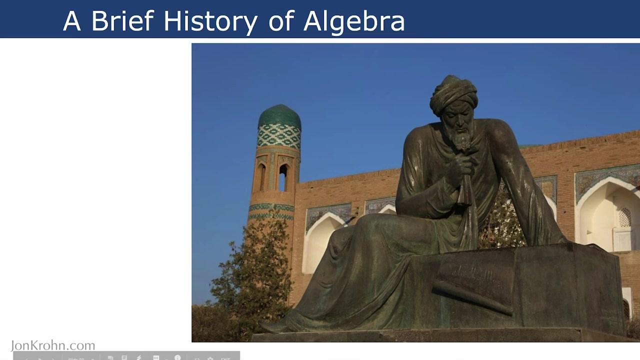 many-dimensional convolutional objects that are specified by these, and these allow for some especially powerful machine vision models called convolutional neural networks. anyway, just want to get you excited about what we can do with linear algebra, these notebooks, these tensorflow notebooks, show you an end point that we're working towards in the series. for now, we'll focus on the fundamentals. speaking of fundamentals, I find it absolutely fascinating to consider the origins, or originり. 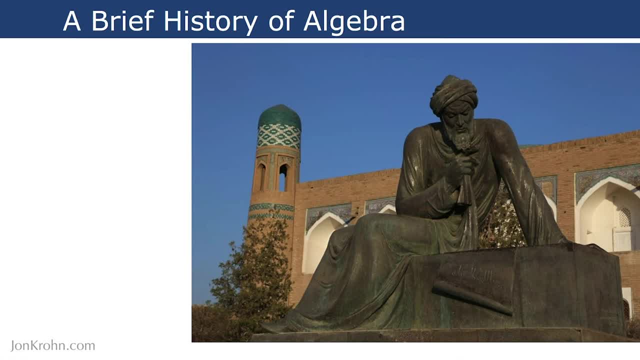 fundamentals. I would certainly like to talk about them now, as I'll just be drawing my notes. after this series of 사라 바수�pendLOD won't be enough to cover of algebra, So let's take a quick moment here to do that. This guy here is Abu Jafar. 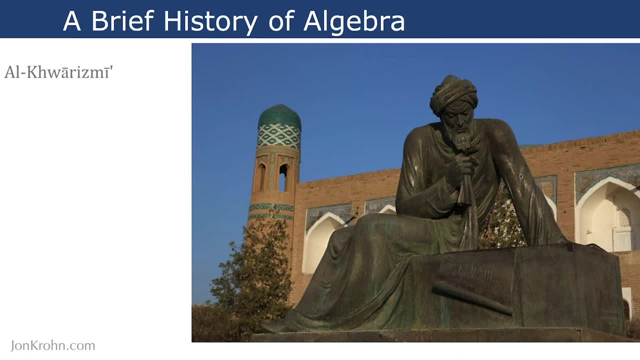 Muhammad ibn Musa, more commonly known as al-Khwarizmi because he came from a place called so. al-Khwarizmi means the man from Khwarizm, and so this is a former center of Persian culture in modern Uzbekistan, today called Hiva So. 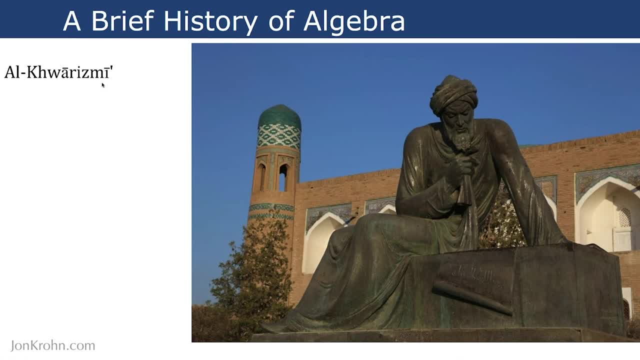 in English we pronounce this al-Khwarizmi. So this medieval Persian mathematician, who was around from 780 to 850 in the Common Era, was not only critical to the history of algebra, as I'll get to in a second, but is also the 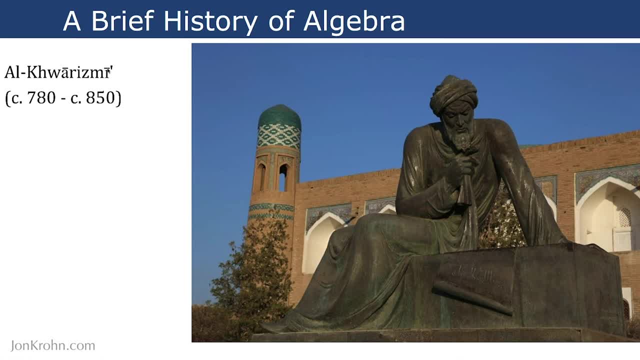 namesake of the word algorithm, So very prominent old mathematician, So al-Khwarizmi, wrote the compendious book on calculation by completion and balancing, And in Arabic this word completion is algebra, So algebra is actually right here in the name of the book And completion and balancing refers. 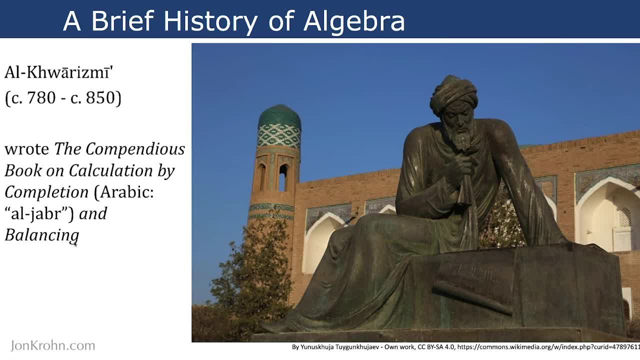 to various ways that we can rearrange algebraic equations, some of which we've already looked at at the beginning of this video. The medieval Islamic Arab Empire made most significant changes in the history of Arabic literature. The most significant changes in the history of Arabic literature: The most significant. 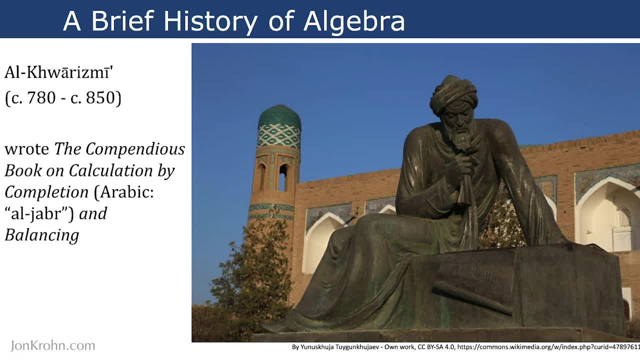 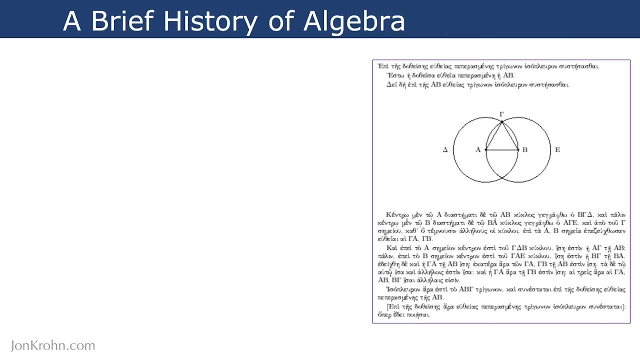 early contributions to modern symbolic algebra. so the kind of algebra that we work with today, Although it was refined significantly by the French, such as René Descartes, in the 17th century. Though, that said, many other cultures developed their own approaches to algebra. So rhetorical algebra, this. 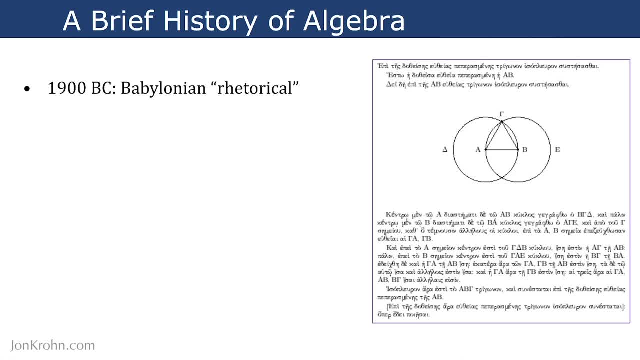 spoken algebra was developed as early as 1900 BC by the Babylonians. There's an Egyptian papyrus which is the most famous one in the world and it's called the Roman papyrus, which is the most famous one in the world and it's called the. 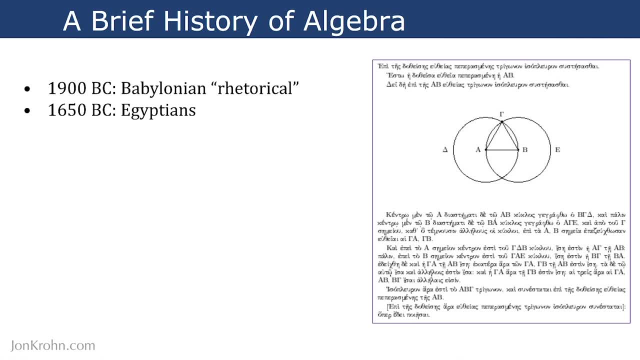 Egyptian papyrus, which is the most famous one in the world and it's called the Egyptian papyrus. And it's not only the European papyrus, but it's also the Roman papyrus. So the Greek people and the African papyrus were customary greatest. 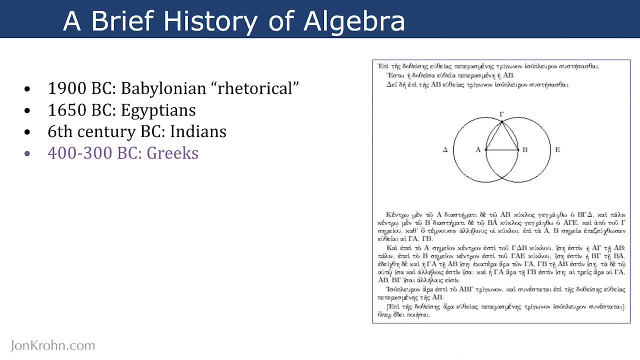 on the Greek territory. So Roman papyrus or other Greek papyrus was the only genealogy that ever existed. So Roman papyrus is an ancient Greek ancientirie. So Roman papyrus is an ancient Greek mixed with the Middle Ages, So it's a word that's kind of related to the Greek. 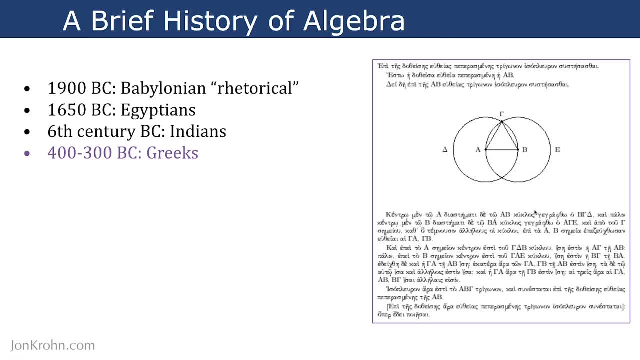 philosopher Plato and is a particular example of this geometric algebra here by Euclid in his book Elements. The Chinese had linear equations solved in a book from 250 BC. This book was called Nine Chapters on the Mathematical Art and although the Europeans started much later, in the late Middle, 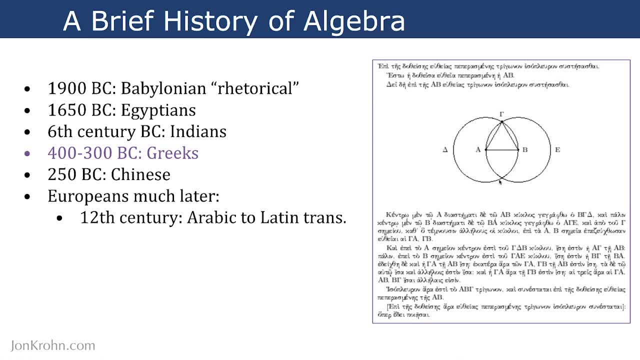 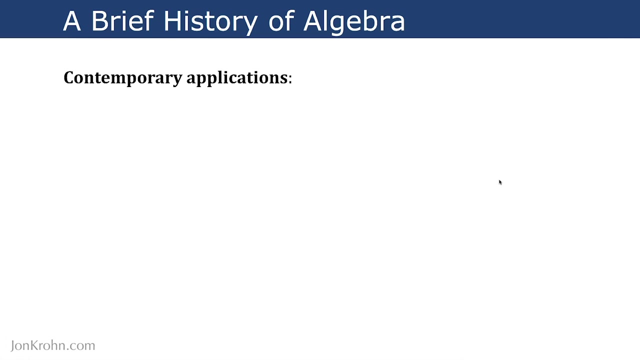 Ages, initially by translating Arabic texts to Latin in the 12th century. by the 13th century, European mathematics rivaled other cultures and when the Islamic empire declined after the 15th century, European culture was left carrying the baton of algebra to today, This technique devised. 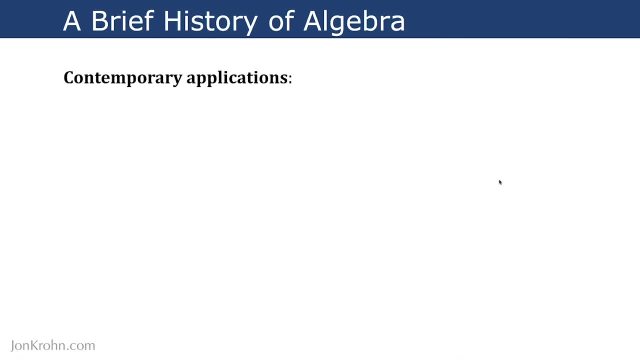 initially, thousands of years ago in some respects, and you can see that it has been used for many, many years In its symbolic form, many centuries ago, by Persian mathematicians. we today have tons of contemporary applications that take advantage of lots of compute power and perform these algebraic 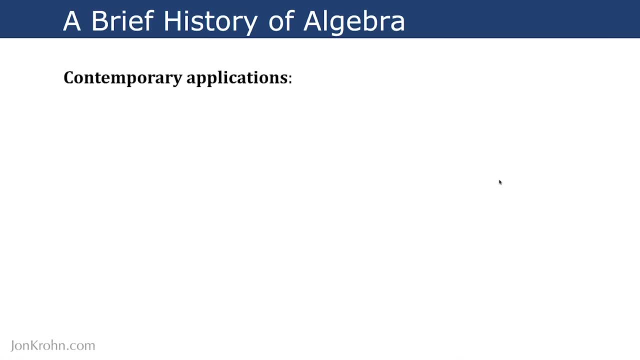 applications in tons and tons of devices all across the world- billions of them, I'm sure. So one kind of straightforward application is solving for unknowns in machine learning algorithms, including algebraic algebra. So this is our primary focus across this Machine Learning Foundations program. 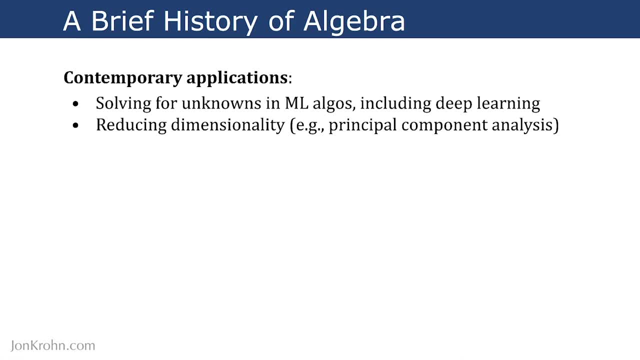 It's also used for reducing dimensionality, so if we have some high dimensional data, we can reduce it down. using techniques like principal components analysis, We can rank web pages in order of importance, For example, with eigenvectors. we're going to talk about both eigenvectors and principal. 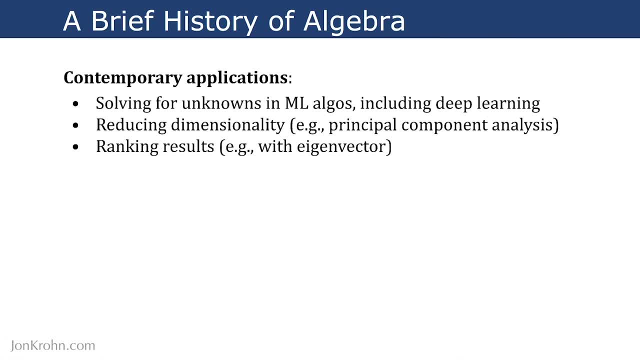 component analysis. in subject to the machine learning foundations program, We're going to talk about the linear algebra 2 of the machine learning foundation series called linear algebra 2.. And same thing with recommender systems. So if you want to build a recommender for movies, for example, based on other movies, 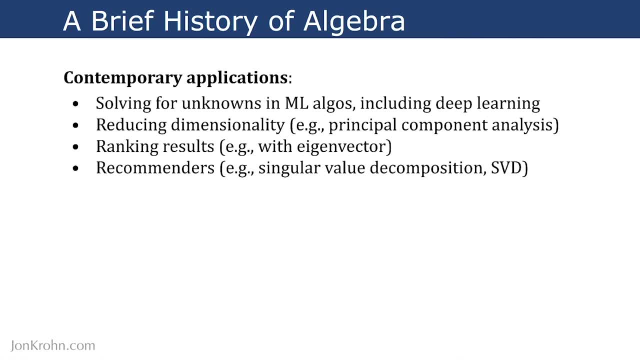 that somebody has watched. you can use singular value decomposition to do that And, again, that is something we'll be covering in linear algebra 2, once we get past the foundational content in this linear algebra 1 course. It's also used to process natural language, you know, with single value decomposition. 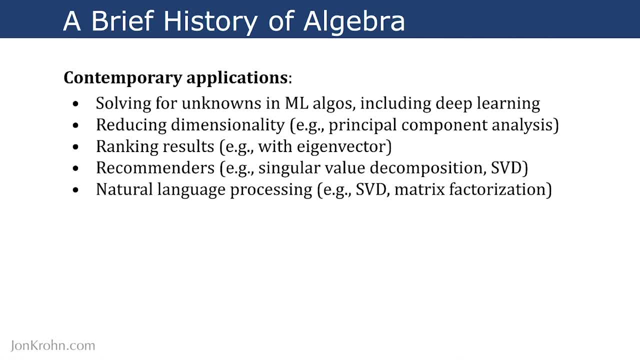 and so on. So, whether we're talking about linear decomposition or another technique called matrix factorization, and so whether we're talking about processing language coming out of somebody's mouth- the language sounds, or written language, we can be using linear algebra to be modeling topics. 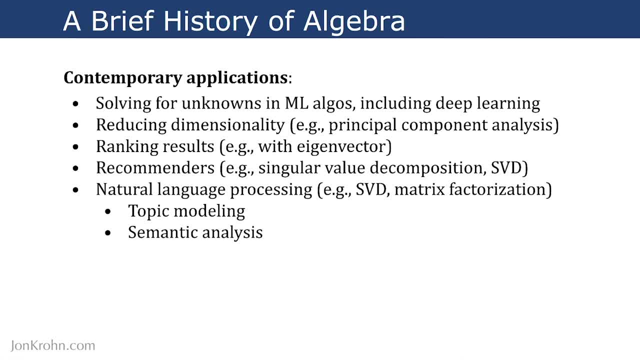 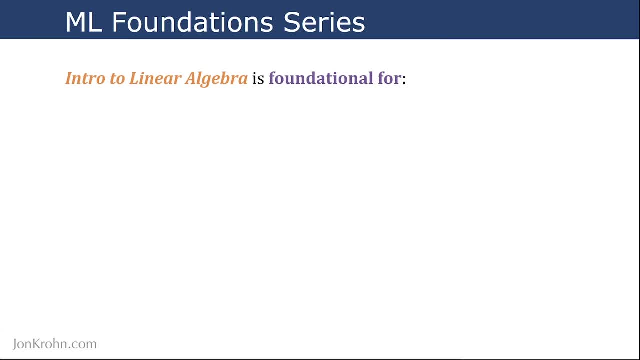 identifying what topics are being discussed in that natural language, as well as for semantic analysis. So in this machine learning foundation series, this intro to linear algebra- subject that we're covering right now is foundational for, of course, the linear algebra 2 matrix operations. 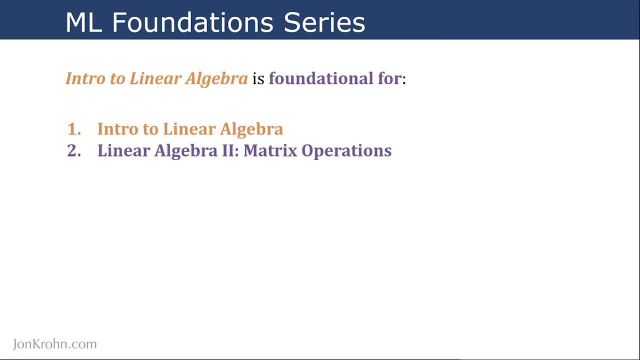 subject that is coming up that will cover eigenvectors in SVD and PCAN. It also- I'm putting it in non-bold here- because it also is foundational for- though not as directly as it is- for linear algebra 2, for our calculus 1, limits and derivatives. subject: 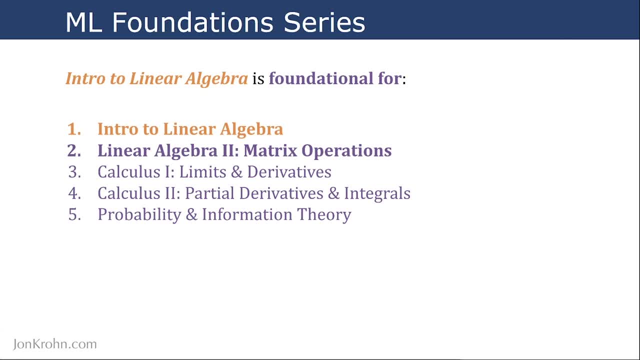 as well as for calculus 2 on partial derivatives and integrals. It's also foundational for probability and information theory and intro to statistics and so on. The only one that it isn't really providing much for is the algorithms and data structures class subject, which is subject 7, and it is very important as basically all of these 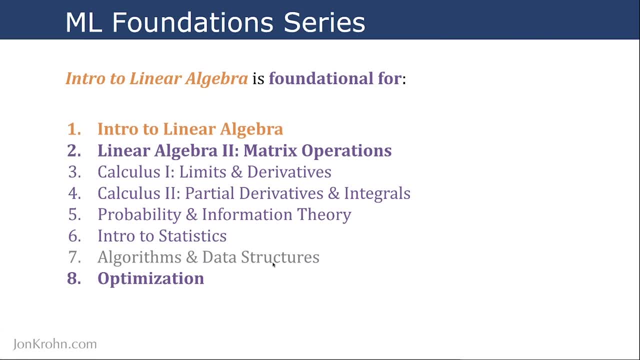 prior 7 are for the final optimization class. that will tie everything together and show us in incredible detail exactly how modern machine learning algorithms optimize All right. Up next, we are going to be introducing All right, We're going to be talking about what tensors are. 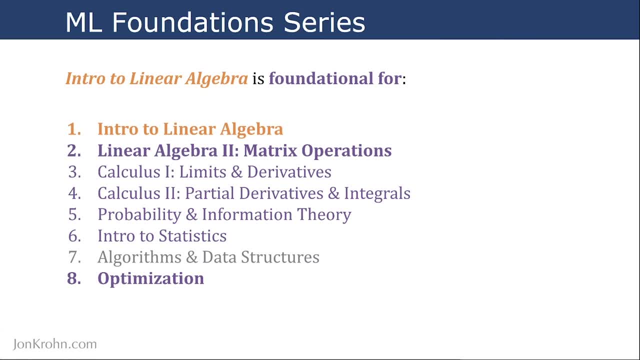 I've mentioned them a few times. We're going to dig into exactly what they are in the next video. See you there. To be sure not to miss the next tutorial in this series, subscribe to my channel. Thanks for taking part in this tutorial. 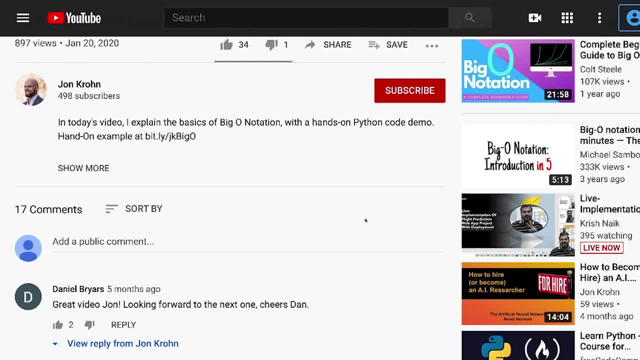 I hope you enjoyed it. If you did, please like and comment To be sure not to miss any of my content. head to johnkrohncom and sign up for my email newsletter. You're also welcome to add me on LinkedIn, Facebook and Twitter. 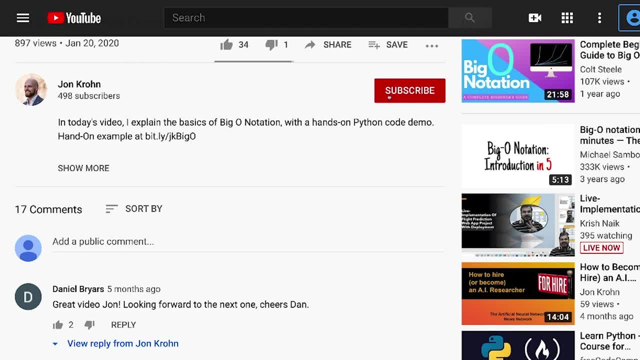 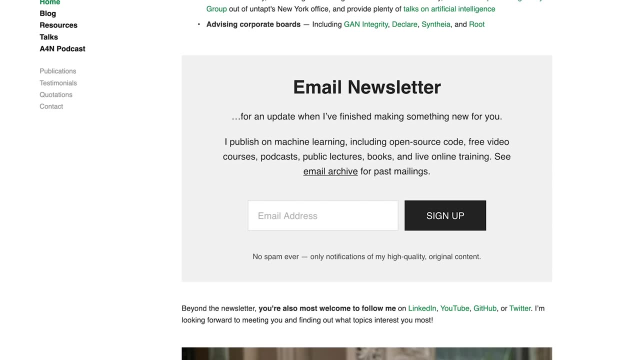 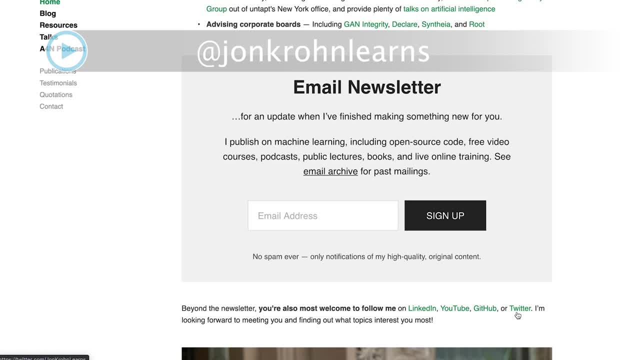 Bye, Bye, Bye, Bye, Bye, Bye. See you next time.